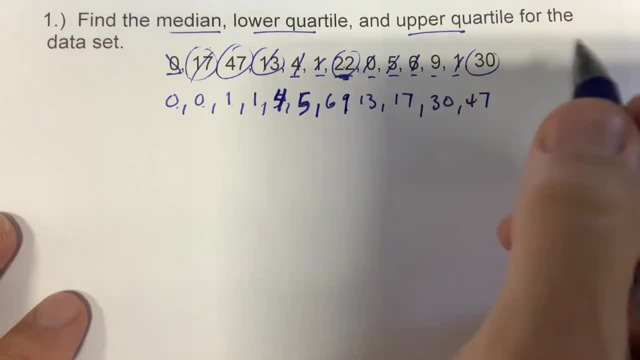 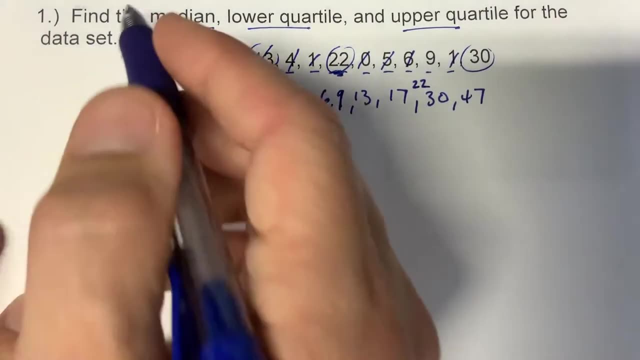 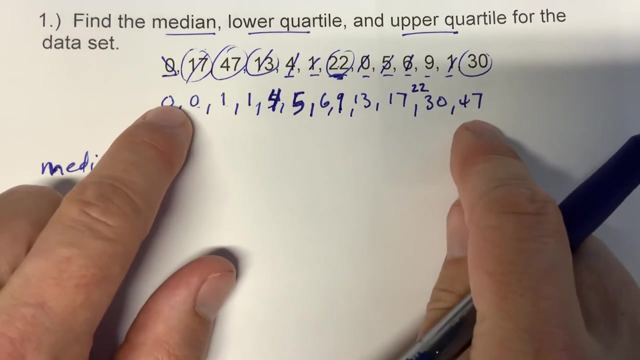 in there, Oh, and 22. 22. That's why we go back and check. Okay, Now, the first one is easy: The median. The median is half of the data. Okay, so I'm going to start at the first and last number and work my way. 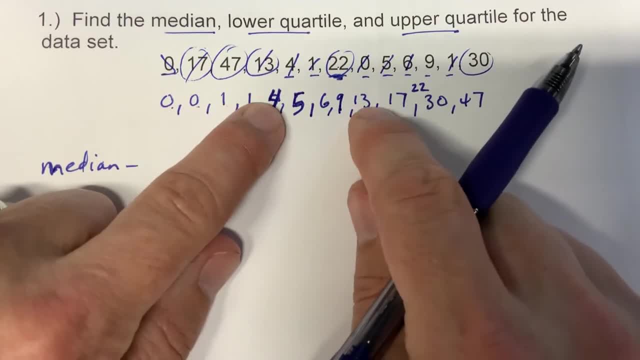 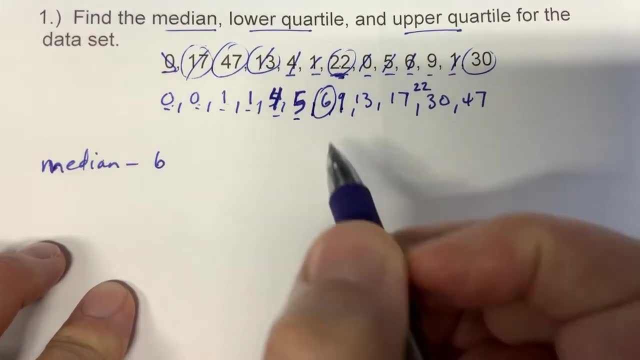 in until I get to a number in the middle, which is six, And I can check by going: 1,, 2,, 3,, 4,, 5, 6. numbers on the left. 1,, 2,, 3,, 4, 5, 6 numbers on the left. 1, 2,, 3,, 4,, 5, 6. numbers on the left. 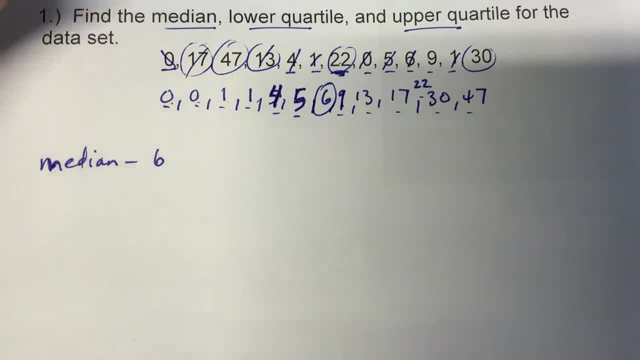 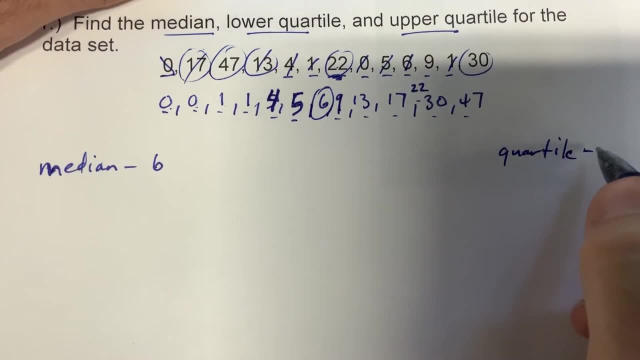 1,, 2,, 3,, 4,, 5, 6 numbers on the right. So yeah, I got my six in the middle. Now we're going to be dealing with a quartile, which is also just as easy. A quartile is one-fourth of the data, So if 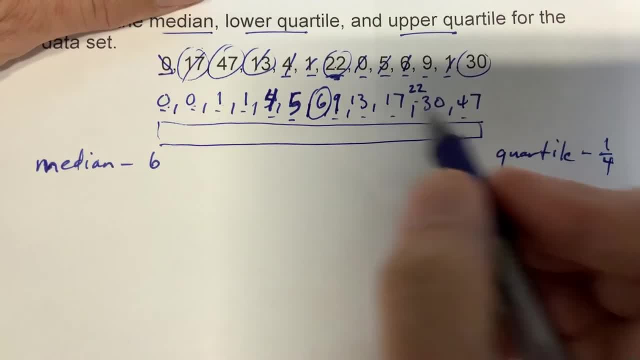 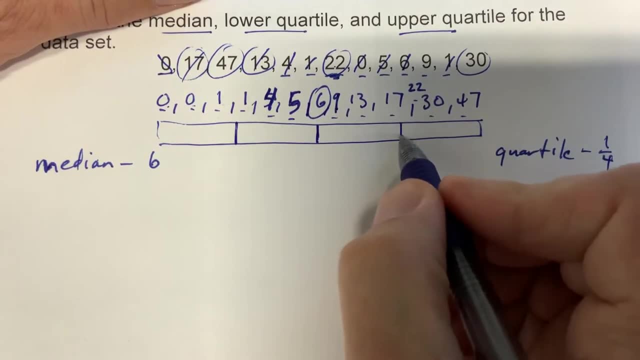 you think of it in terms of like a drawing, the median is going to be right in the middle right. Medium means middle Quartile is one-fourth of the data. So if I divide this data into four pieces, this is going to be the first quartile. 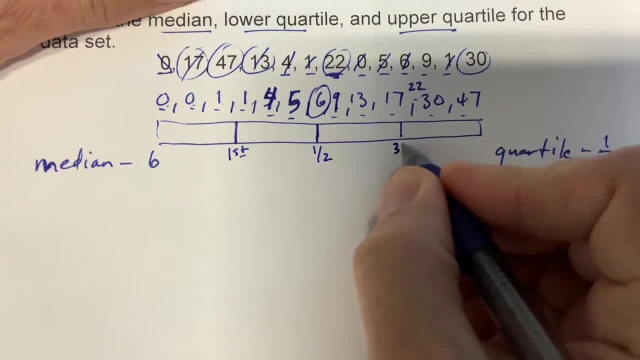 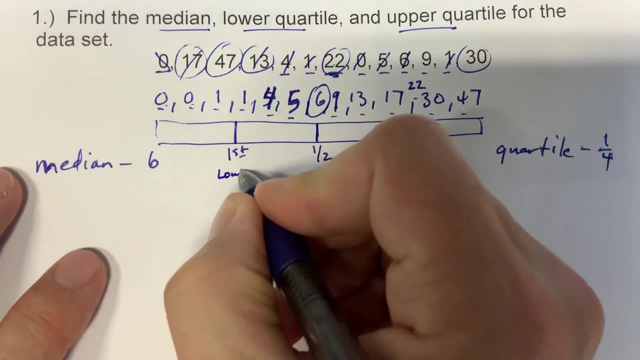 This is going to be the halfway point, or the median, And this is going to be the third quartile, okay, or the upper quartile. So the first quartile is the lower quartile, The third quartile is the upper quartile, And we're going to do the same thing that we did to find the median for the 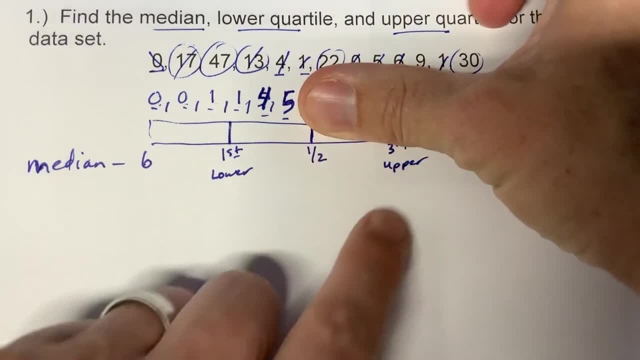 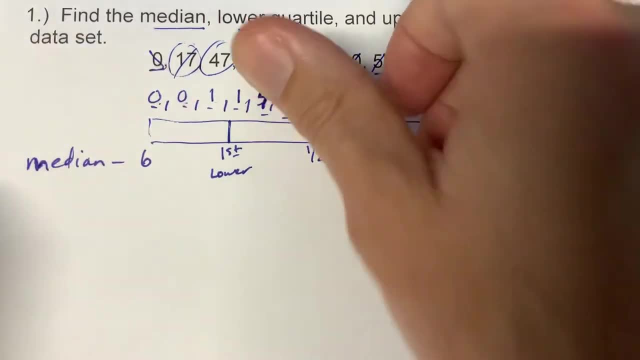 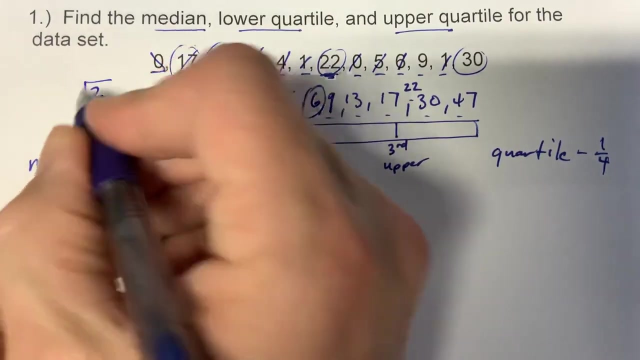 quartile. We're going to cover up all the data, that's the median and everything bigger, and find the middle here. So I point to the biggest and smallest and I move in and I see I have two numbers in the middle. Whenever you have two numbers in the middle, you add them. One plus one is two And then you divide by how many. 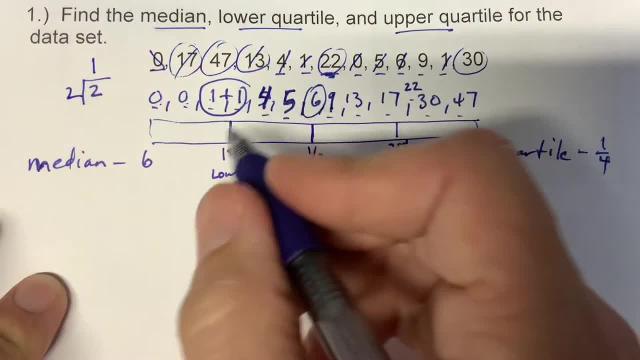 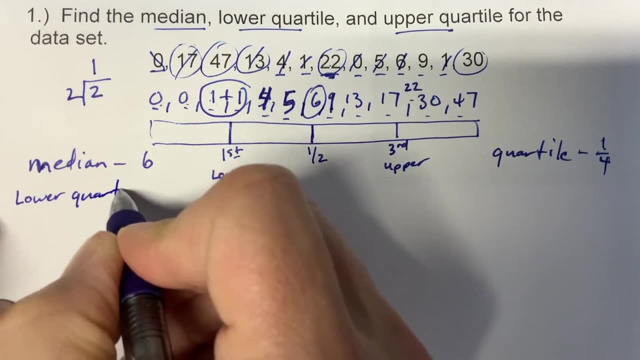 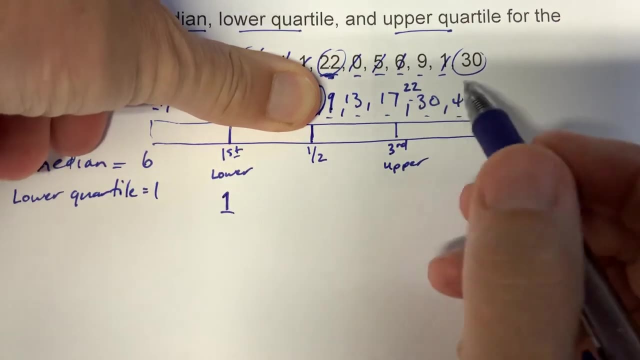 numbers you added We've divided by two numbers. Two divided by two is one. So the lower quartile is one. Lower quartile is one, The upper quartile- I'm going to do the same thing: Cover up all the numbers smaller than the median, point to the biggest and smallest and move in one number at a time. So 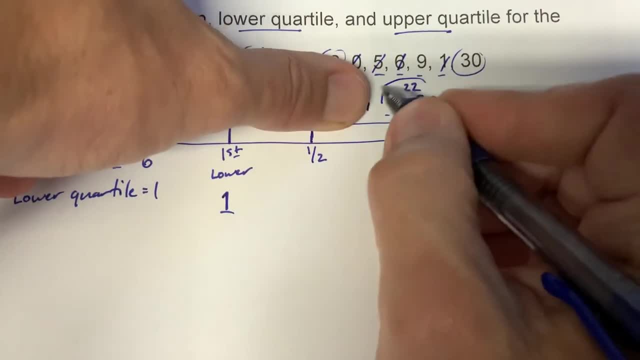 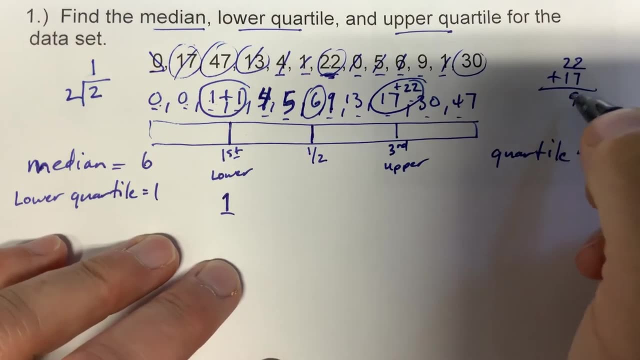 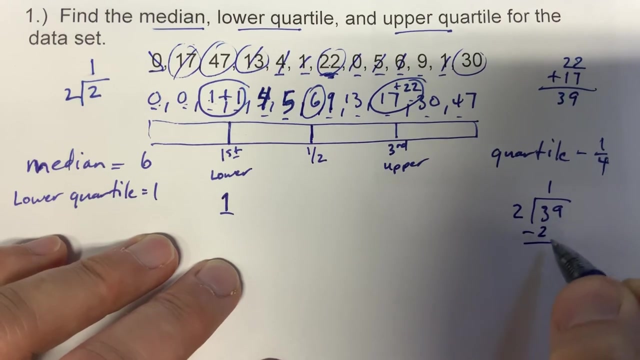 there we go, There we go, There we go, And we have two numbers in the middle. again, I'm going to add those two numbers: 22 plus 17 is 39. And then I'm going to take 39 and divide by two, because I added two.